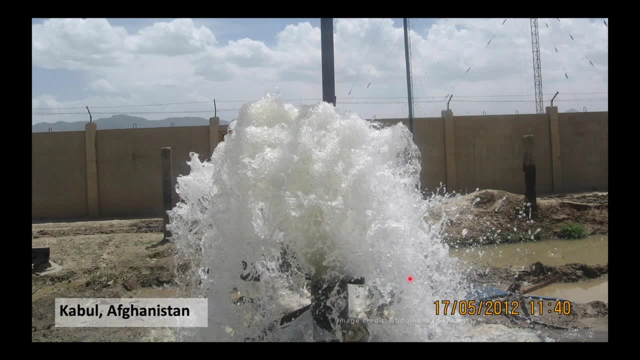 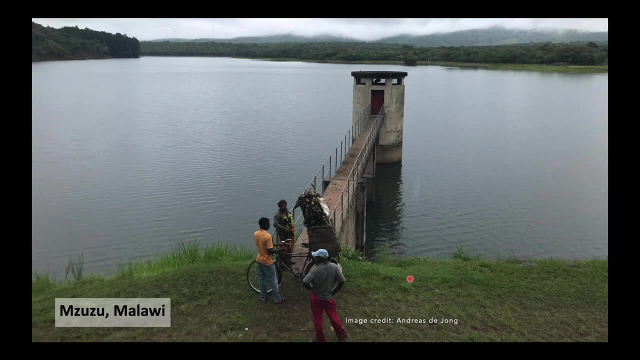 so congratulations to the Afghan engineers who drilled this well in Kabul. There is a problem, however. Surface water is always easy to find- You can see it with your own eyes- whereas groundwater is mostly invisible. and if we want to look for it? 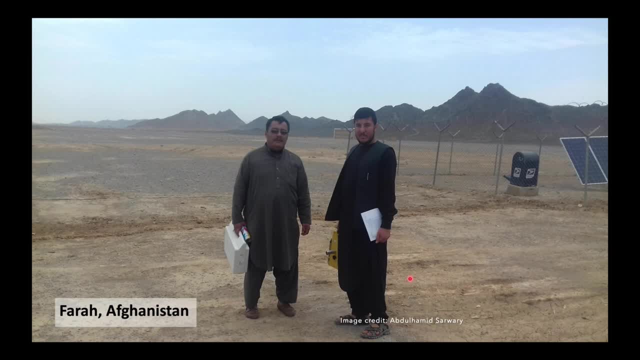 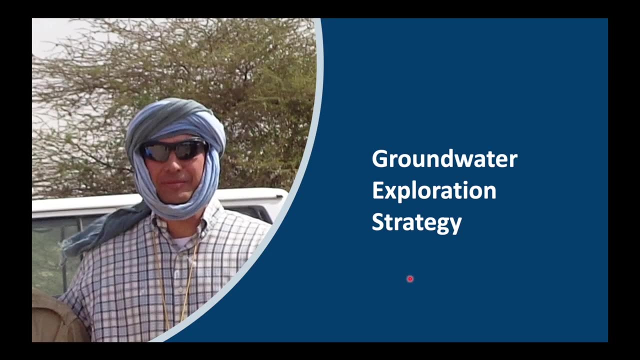 it costs us a lot of time and, more importantly, a lot of money, because we have to drill in order to verify if it's there or not. My name is Andreas de Jong and in this short video, I'd like to talk about my preferred groundwater exploration strategy. 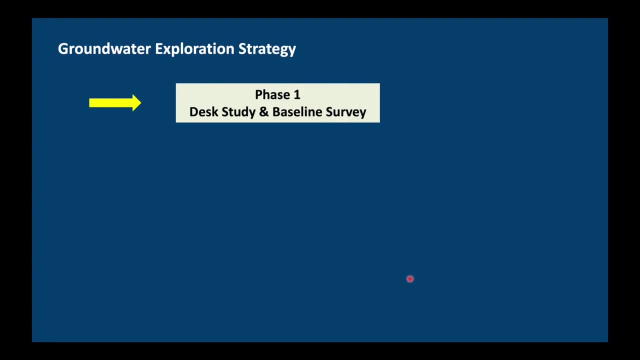 We should split every groundwater exploration project into a number of distinct phases. The first phase is the desk study and baseline survey. It's not that expensive and at the end of it we can decide whether we stop the project, proceed with caution or give it a green light During the desk study. all we want to do is to 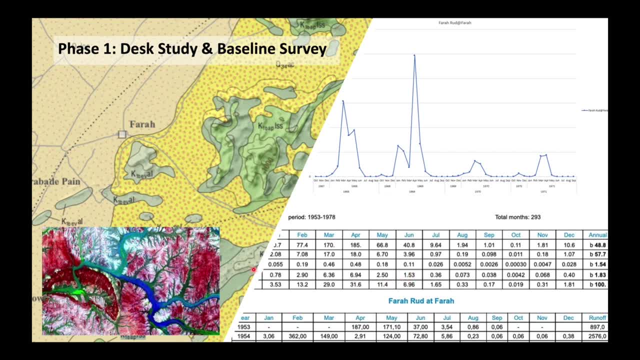 collect as much information as we can about the project area. so that includes the geological maps, maybe some satellite images and any information whatsoever to do with water resources, so not just water. If there is information on groundwater, great, but don't forget your surface water flows. 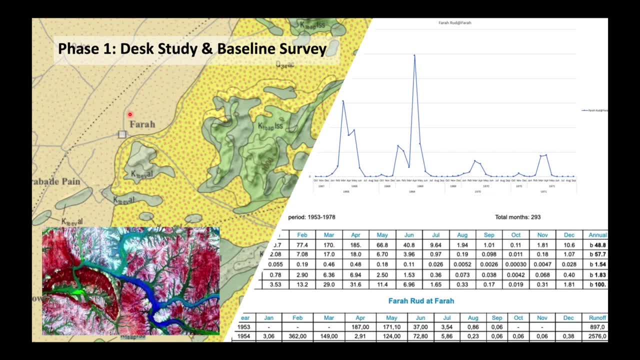 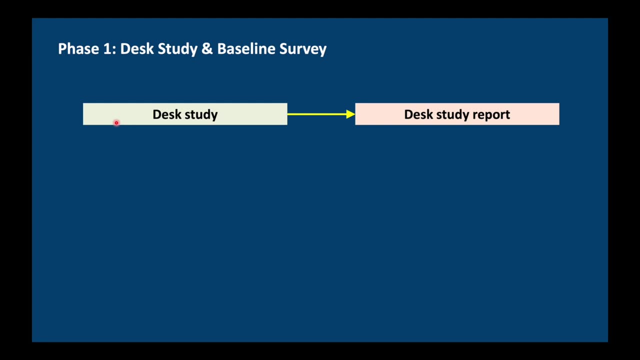 precipitation and so on, because we don't just want to find the right place to drill the water well, we also want to look at its long-term sustainability and effects of climate change. Our desk study will result in a desk study report where we put everything into a neat little report. 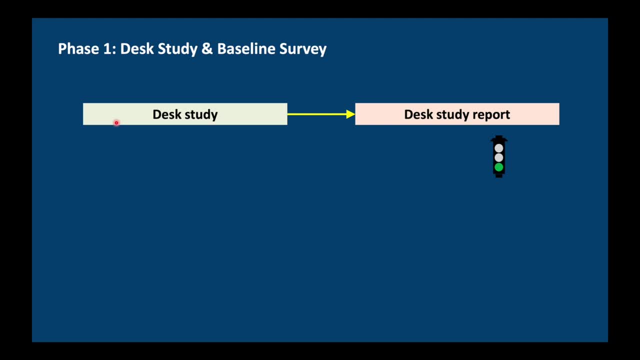 which will decide for us if we want to continue with the project or not. If we continue, it's usually a good idea to carry out a baseline survey. Sometimes the baseline survey is done at the same time, or maybe even before the desk study. it just depends on your. 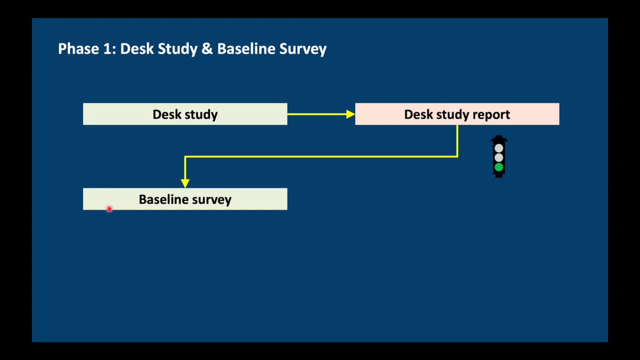 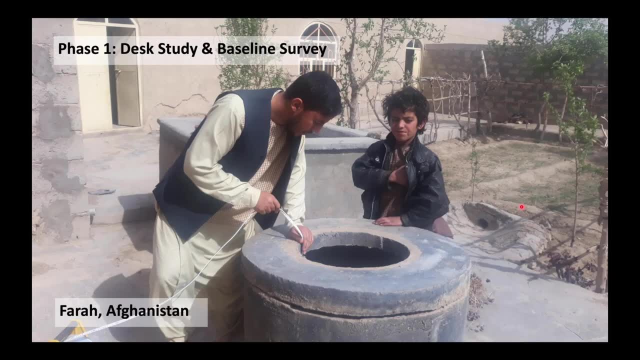 project and doesn't really matter, but it is important to carry out a baseline survey because most of the data that we use in a desk study is usually out of date. During the baseline survey, we want to visit as many different water points as we possibly can. the more the better. So all these 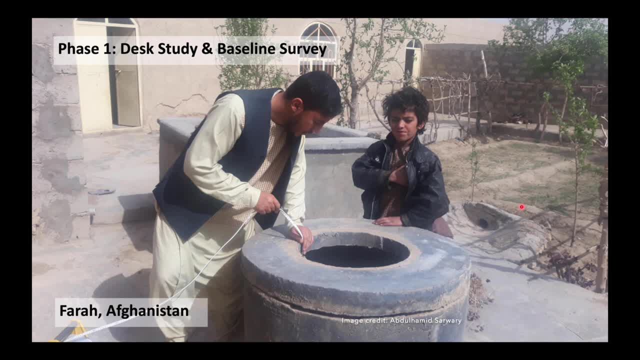 existing wells. you need to know how deep is the static water level, get some idea about water quality, maybe measure the electrical conductivity, maybe take some samples. but most important of all is to talk with the well owners. Ask them, when they drilled the well, how deep was. 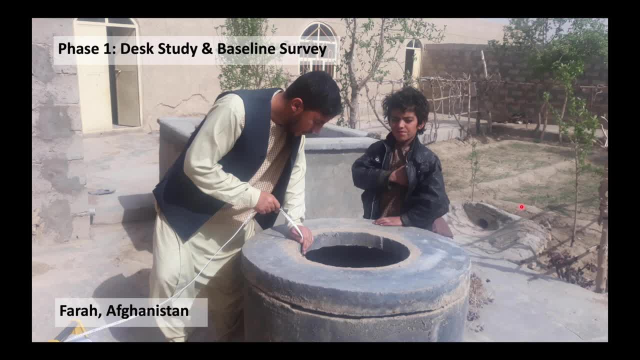 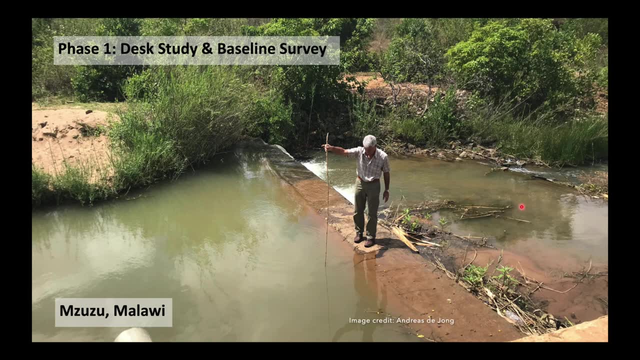 it? has there been any problems over time in terms of quantities or qualities? Don't forget to look at surface water resources as well. In this stream here, which is in the dry season, we can see it's sustained by groundwater, So we can always think about not just groundwater, but also the whole. 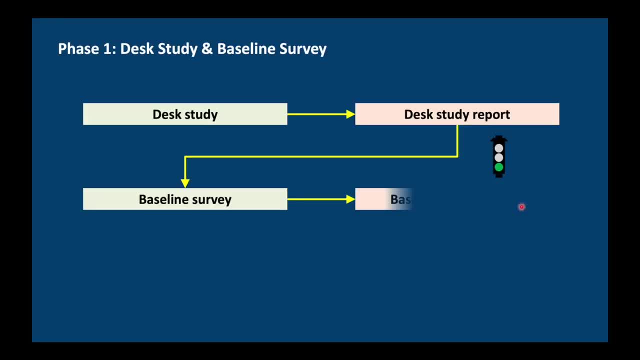 water cycle when we look for groundwater. Now, our baseline survey will result in a baseline survey report. It doesn't have to be anything very elaborate. this could be just a series of maps and some tables, which is then part of our desk study report, But basically what we want to do. 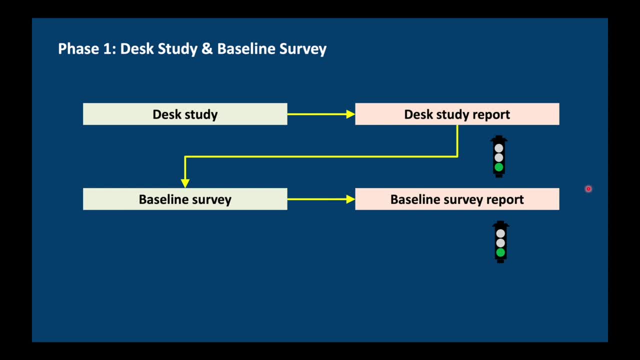 is again to decide whether the project goes ahead or not. If we have a green light, this is the time when we design our geophysical survey and we write the geophysical tender documents. We need to know where are we going to look for groundwater, how deep should be the? 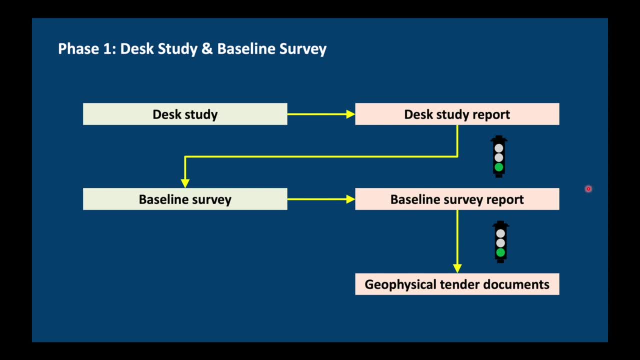 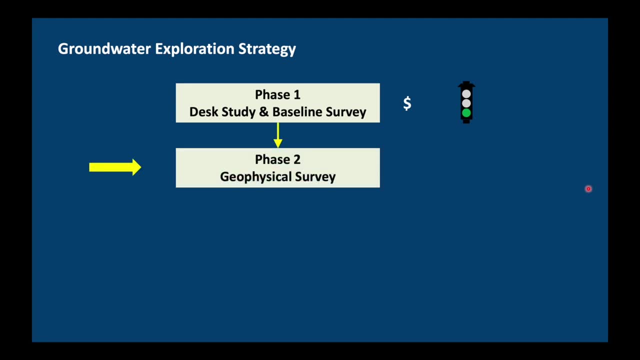 depth of investigation, how many locations should be surveyed, and so on. So let's assume that our phase one is completed successfully and we're now going to do phase two, which is the geophysical survey. The geophysical survey is a little bit more expensive. 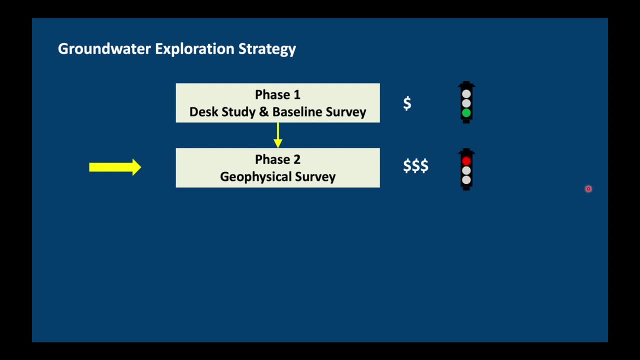 but at the end of it we can decide whether to stop the project, to proceed with caution or to give it a green light. So this is advantage of the phased approach of groundwater exploration: At any point we can stop the project if we think that the risks are too high. 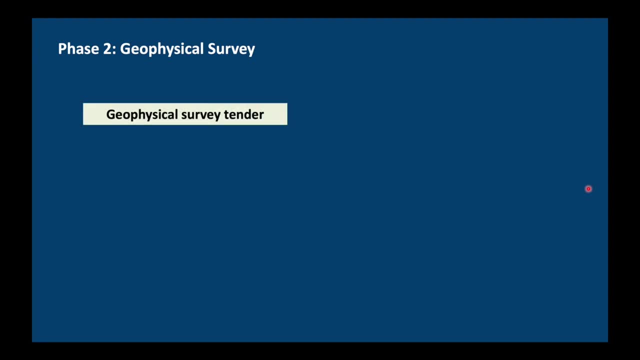 Now we've written our tender documents previously. now we're going to launch the geophysical survey tender and again, before we award it to a contractor, we have to make sure that this person or company is actually able to do the geophysical survey. If we just award to the cheapest contractor and they do a rubbish job, basically our whole. 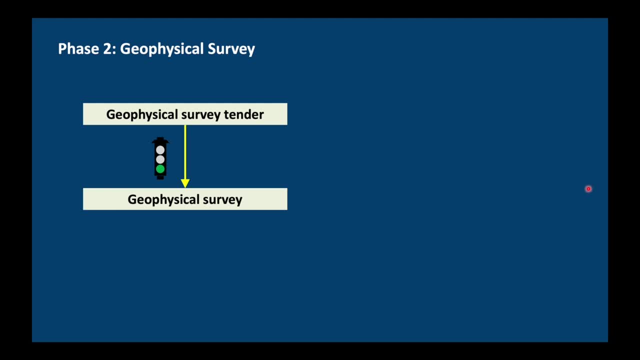 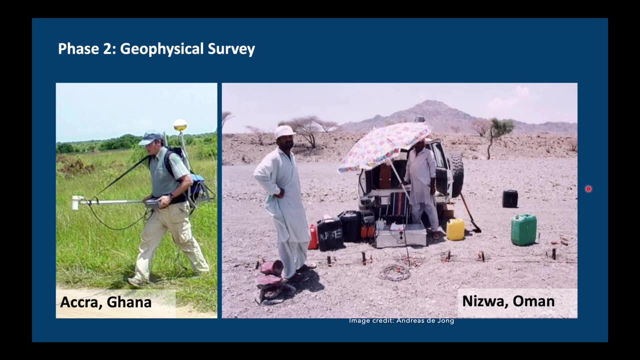 project will fail. So it's very important that we select the right people to do the job. Sometimes, the right people is ourselves. So here is an example of me doing a magnetic survey in the plains of Accra in Ghana. Here is a more traditional resistivity survey in one of the wadis near Nizwa in Ghana. 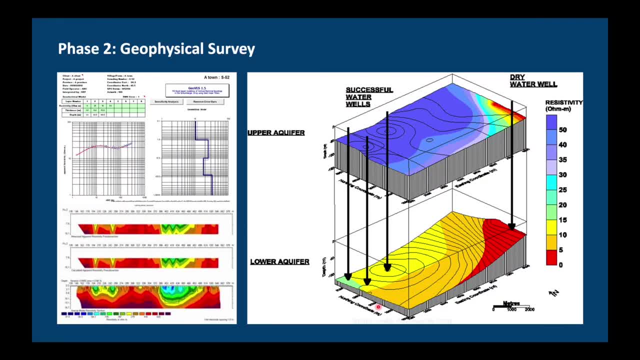 Oman, and once we finish the geophysical survey, we're going to interpret the data, and it's very important that our geophysical survey is designed in such a way that we can work out what is the depth of the aquifer and also how it changes over distance, so that we can select the correct places to do our 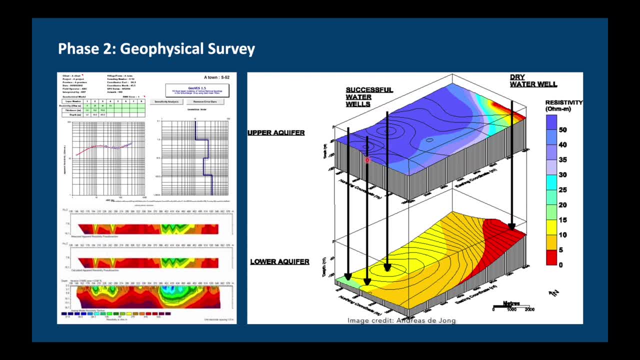 drilling and also to know how deep the well should be. This is an example from the Balochistan desert of Pakistan, where an existing well was drilled here. in fact, two wells were drilled here. they were both dry, and then, following the geophysical survey, we saw that the resistivity increases towards the 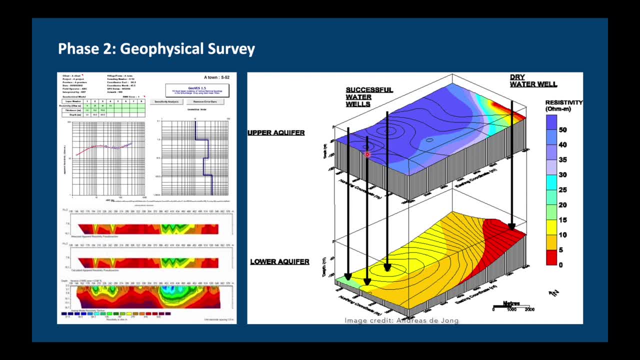 northwest. so we located three drill sites. all were successful. Example here is from Ghana. we're looking for a fracture zone and we managed to find it here from our geophysical profiling and we did a VES which showed that also here the weathering is down at about 80-90 meters. so we drilled. 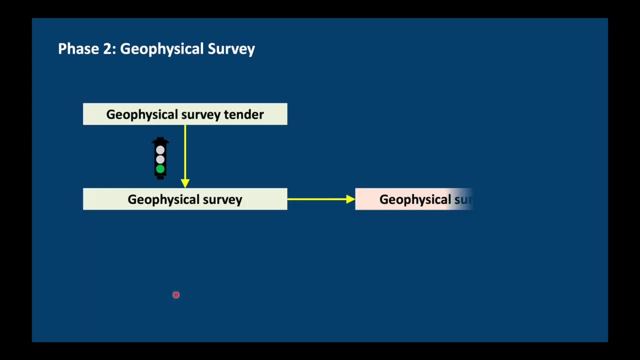 away and we found that the geophysical profiling was not very good, So we did a well here, also successful. Now the geophysical survey should result in a geophysical survey report, usually written by the geophysicist, and if it looks successful, then we move ahead and use the geophysical survey information. 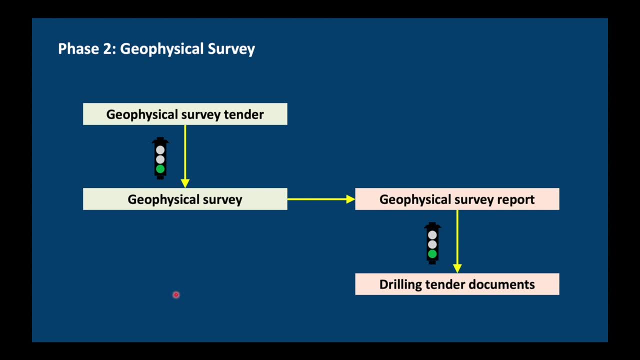 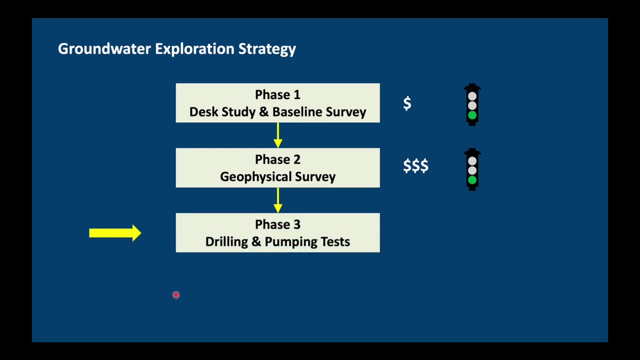 to write the specifications for the drilling tender documents. By that I mean how many wells should be drilled and how deep. So the well depth is not some kind of speculation. it is based on the results of the geophysical survey. Okay, so our geophysical survey has been. 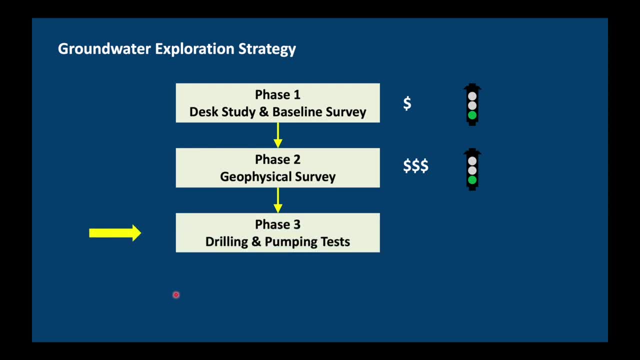 successful. We're now moving on to phase three, drilling and pumping tests. This is the most expensive part of groundwater exploration and often all people look at is this budget here and they want to move ahead with this as fast as possible and they want to ignore these study phases. 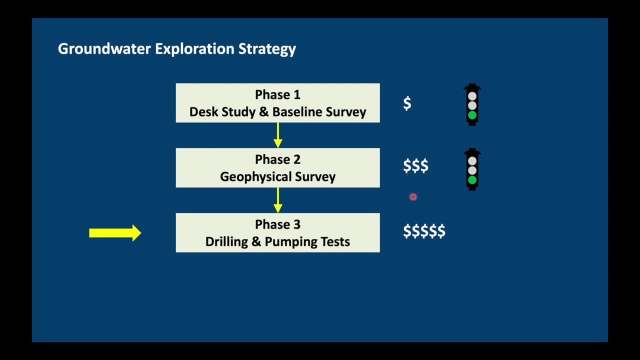 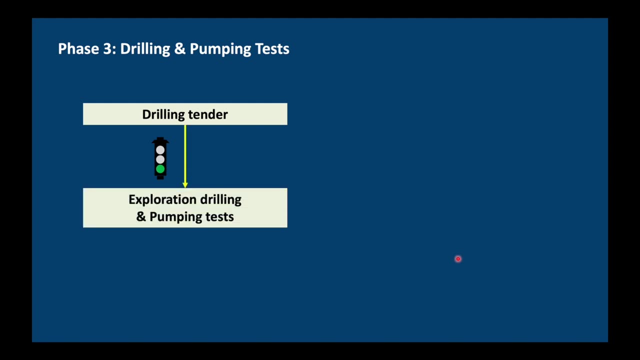 The baseline survey, desk study and geophysical survey. but actually we have to do this. We have to be very careful that we do a good job before we start drilling, to reduce the chances of not drilling successful wells. Okay, so we launch our drilling tender and, if everything is okay, we will award it to a drilling 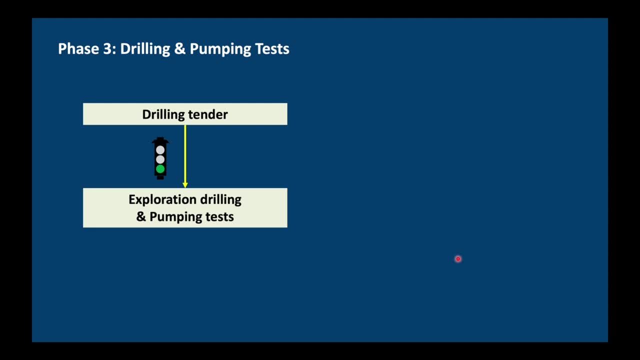 contractor. Now, do not be afraid to not award this tender. If you don't have a good contractor, don't go ahead with the project. You can always re-tender your drilling until you have the right company, the right person, to carry out the. 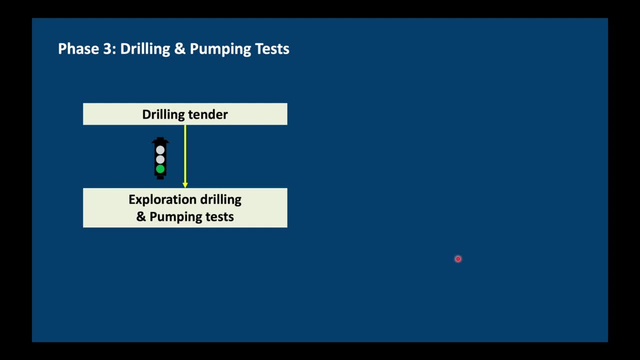 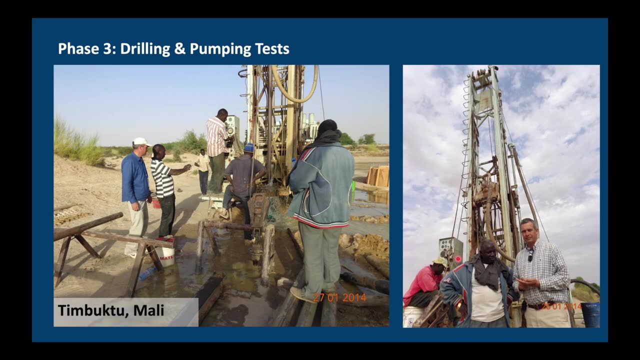 drilling, Because if you don't have a good drilling contractor, they're going to mess up your wells and you will not have a successful project. Here are some pictures more from Timbuktu in Mali and at this stage of the project, the most important person of the project- it's not you- is this guy here, the. 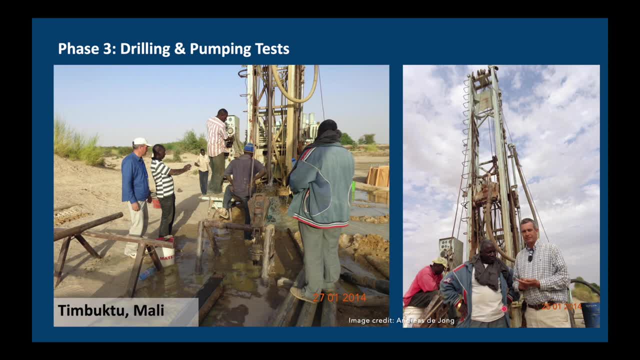 driller, Because if you have a good driller, he is going to do what you ask him to do and drill some good wells for you. If you have a bad driller, he's going to mess up your wells, They'll collapse and he'll say: there's no water and the project will fail. So 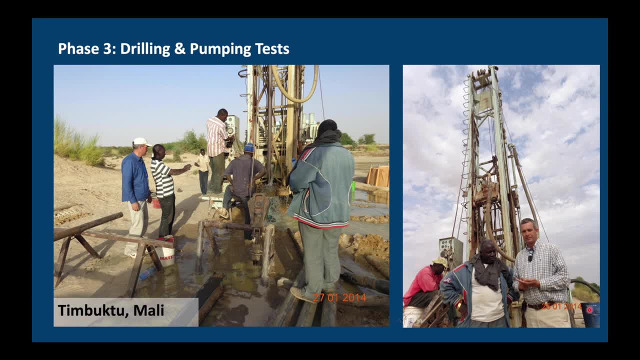 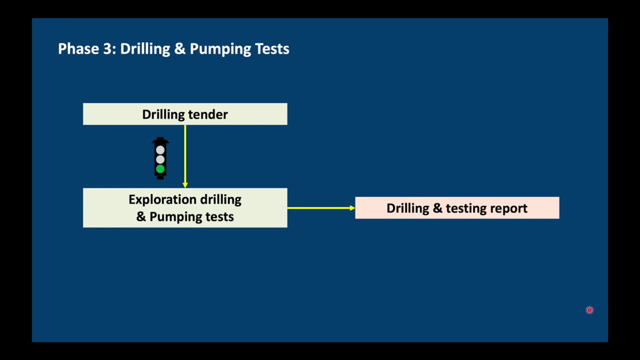 show some respect for the driller and make sure you establish a good relationship with him. Okay now, the output of this drilling and pumping test is a report which is usually written by the drilling contractor. Now the report will contain all the data from the drilling and testing, but the interpretation, of course, has to be done. 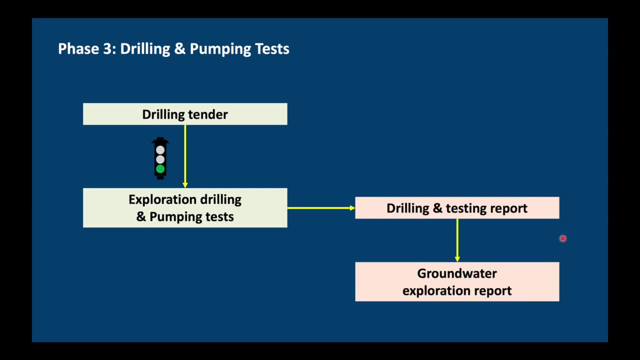 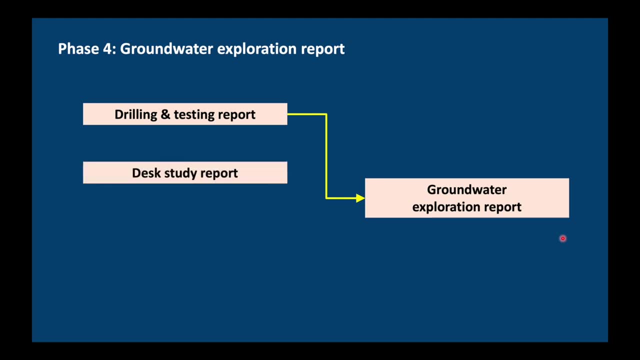 by you, the hydrogeologist, And that's usually done in what I call a drill test. It's usually done in what I call a ground water exploration report. So that report will contain not only all the drilling and testing data, but also information from 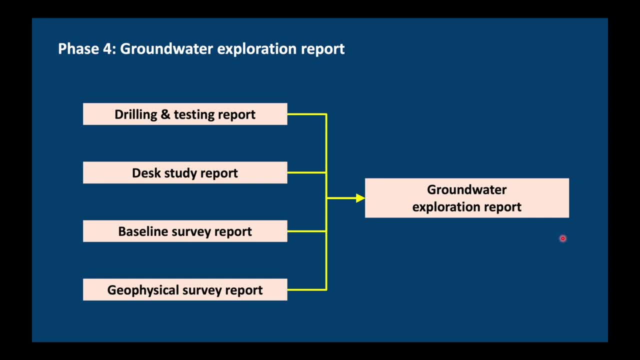 the test study, the baseline survey- if you've done one- the geophysical survey report and finally, you want to do a bit of analysis as well, to look at aquifer sustainability, reach operates and so on. Sometimes it is justified to do modeling, but I would say that's only really important if we're designing a well. 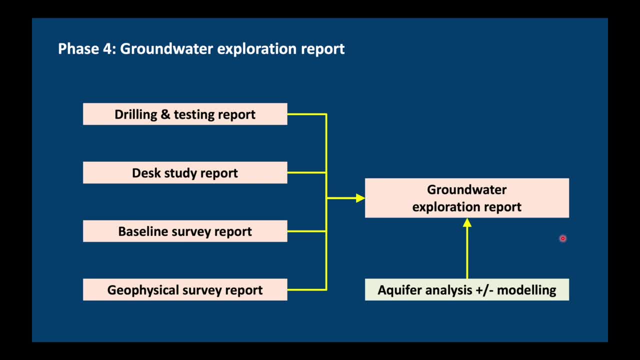 field. For most of us, it has to be a well field. We do know that, but it's only really important if we're designing a well field for most of the time. So this is one of my main ones: projects you don't have to do modeling, Okay. so what I'd like you to take away?